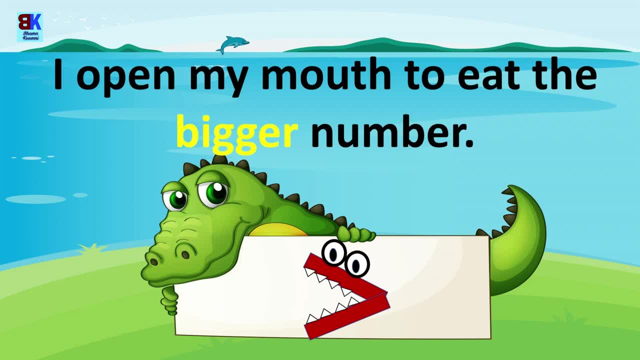 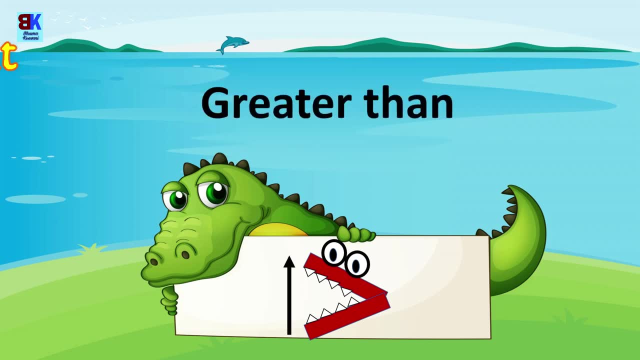 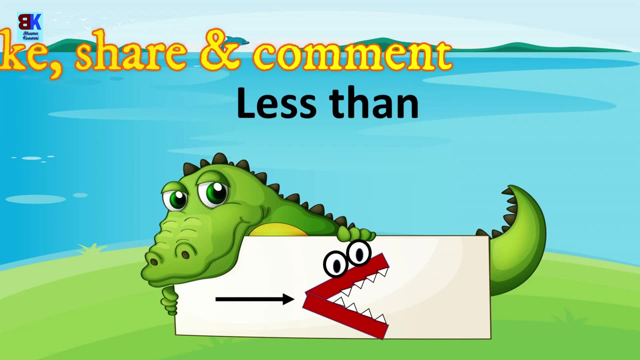 Remember that I open my mouth to eat the bigger number. This is the concept of greater than, less than and equal to. This is the greater than sign where I open my mouth to eat the bigger number. This is the less than sign where the back of my mouth points towards the smaller number. 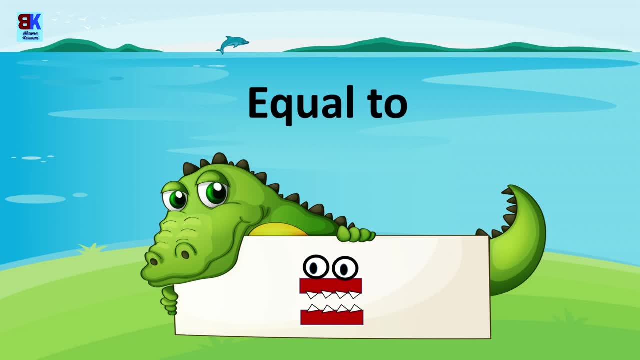 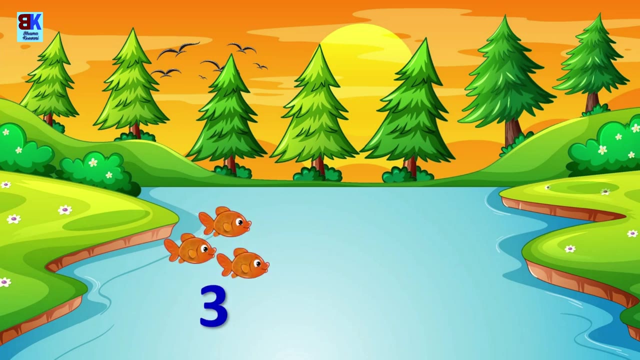 And this is the equal to sign where numbers on both the sides are the same and hence equal. Let us see the concept of greater than. Let us see some examples. We have three fish and one fish. You already know that three fish are more than one fish. 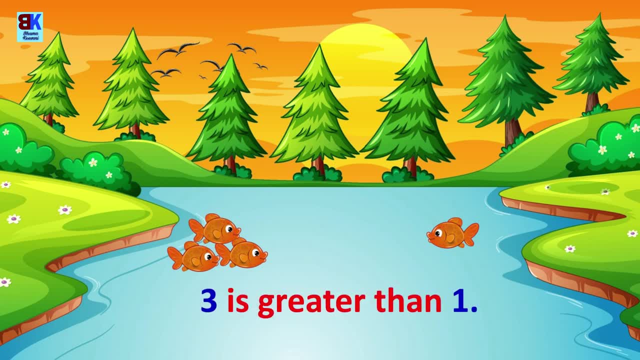 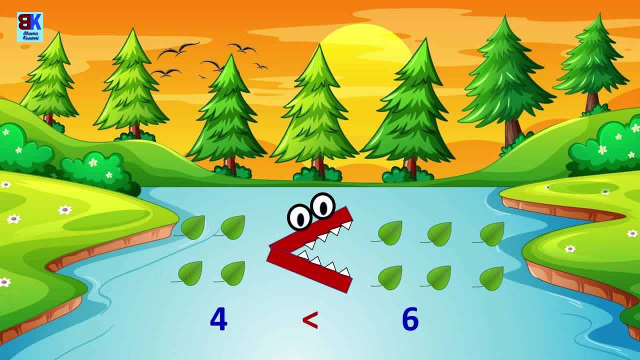 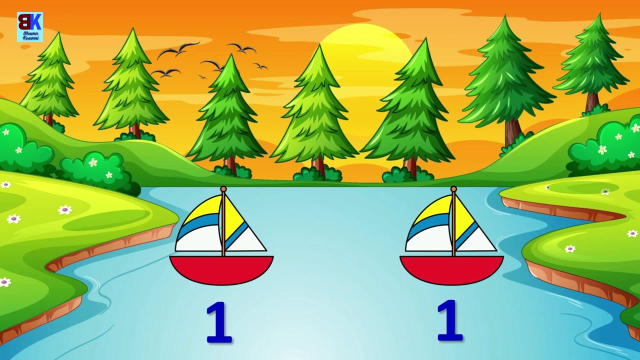 I will open my mouth towards three. I will open my mouth towards three, I will open my mouth towards three, towards the big number six, and the back of my mouth will point towards the small number four. four is less than six. here we have one boat on each sides. that means 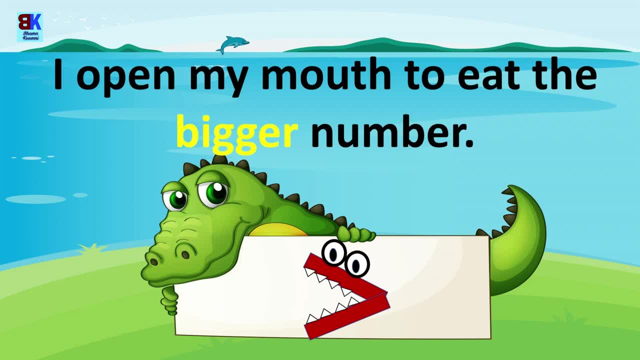 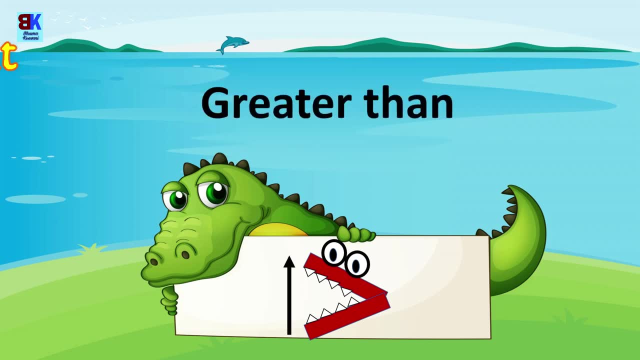 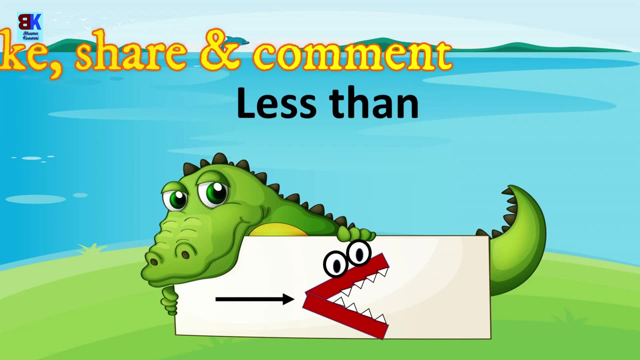 Remember that I open my mouth to eat the bigger number. This is the concept of greater than, less than and equal to. This is the greater than sign where I open my mouth to eat the bigger number. This is the less than sign where the back of my mouth points towards the smaller number. 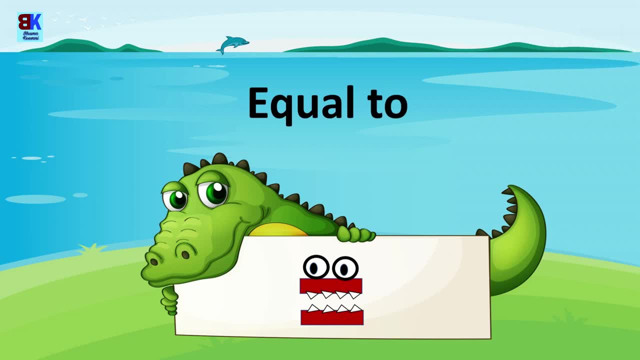 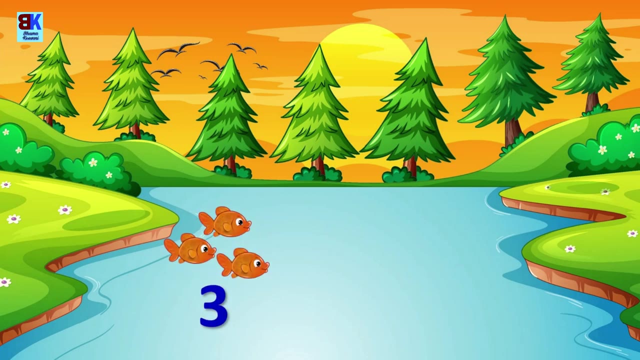 And this is the equal to sign where numbers on both the sides are the same and hence equal. And this is the equal to sign where numbers on both the sides are the same and hence equal. Let us see some examples. We have three fish and one fish. 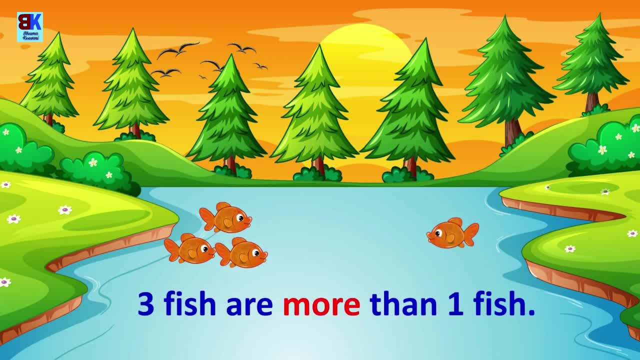 You already know that three fish are more than one fish. In other words, three is greater than one. So where will I open my mouth Towards three because it is greater than one? In this example, we have four leaves and six leaves. 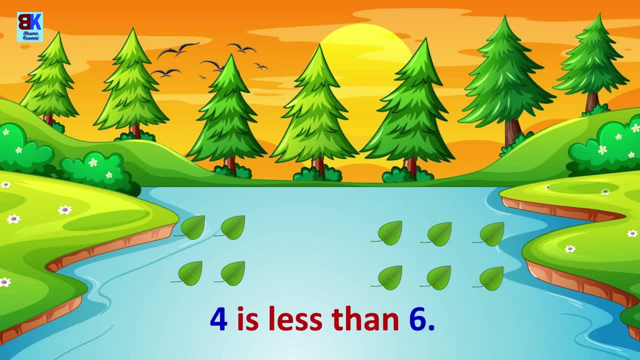 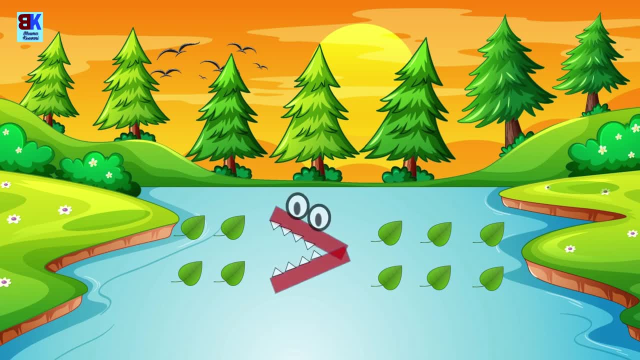 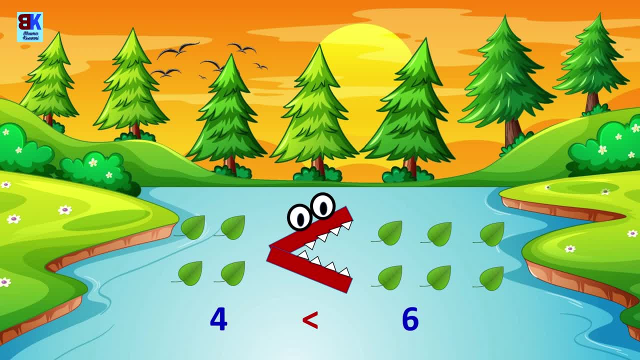 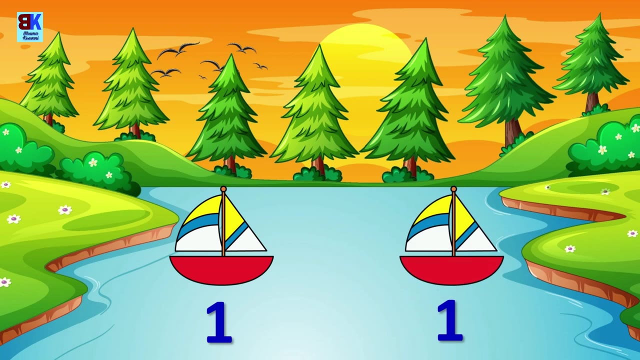 the small number 4.. 4 is less than 6.. Here we have one boat on each sides. That means 1 is equal to 1, as we have the same number on both sides. So let's put the equal to sign here between 1 and 1.. 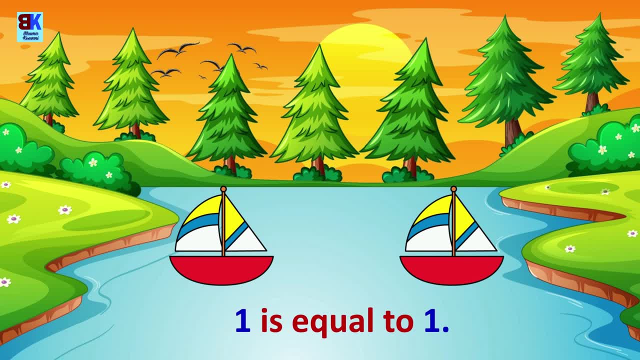 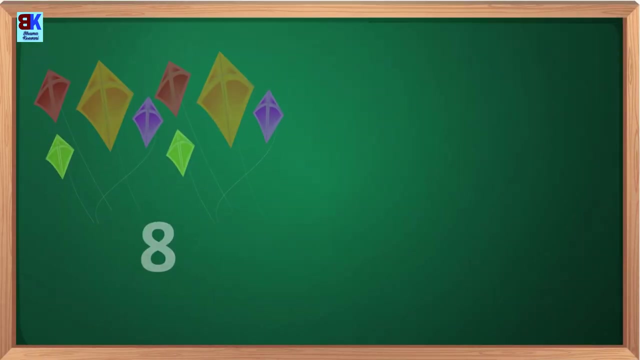 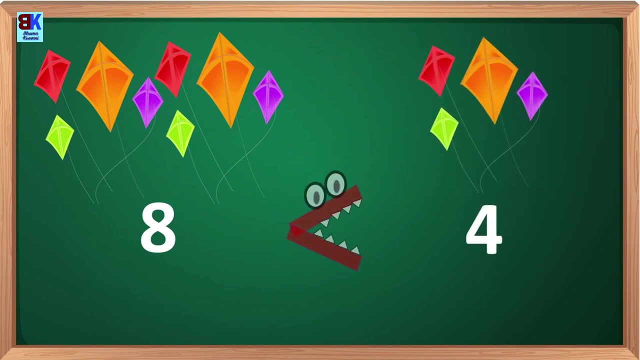 one is equal to one, as we have the same number on both sides, so let's put the equal to sign here between one and one. now your turn. we have eight kites on one side and four kites on the other. that's right. i will open my mouth towards eight, because eight is greater than four. 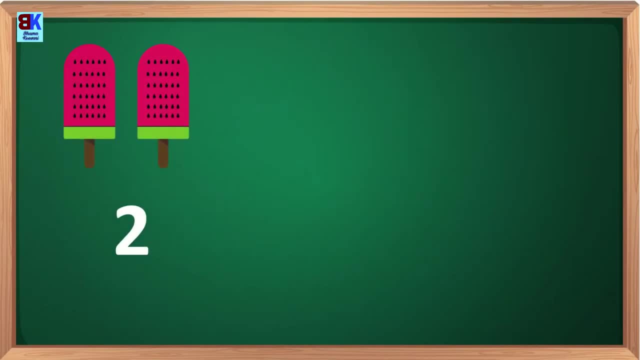 now we have two popsicles and three popsicles. correct, two popsicles and three popsicles. two is less than three, so the back of my mouth will point towards two and i will open my mouth to eat the number three, which is bigger than two. two is less than three. 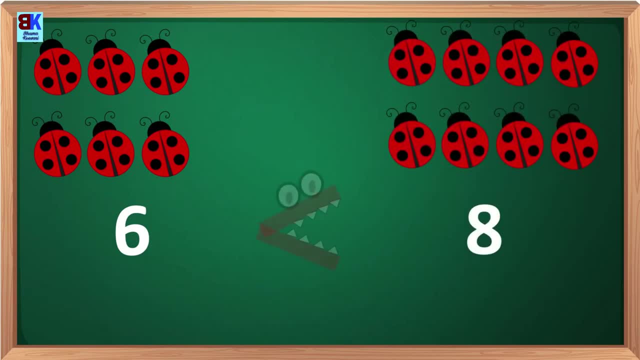 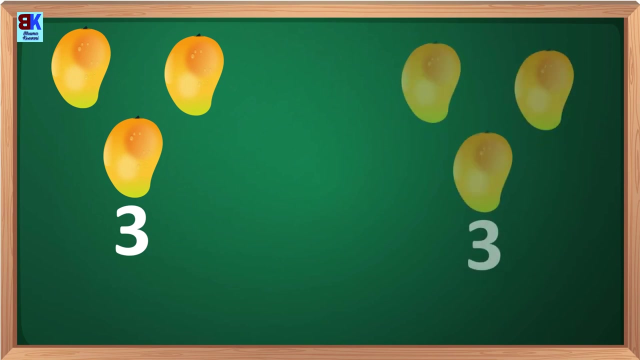 six ladybirds and eight ladybirds. again, i open my mouth to eat number eight and point my the back of my mouth towards six. six is less than eight. three mangoes and three mangoes. so we have equal mangoes on both the sides. three is equal to three. 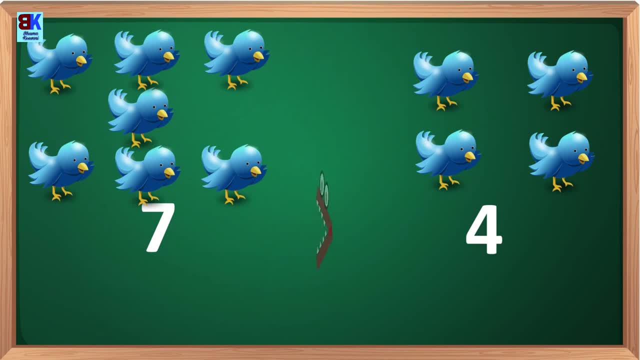 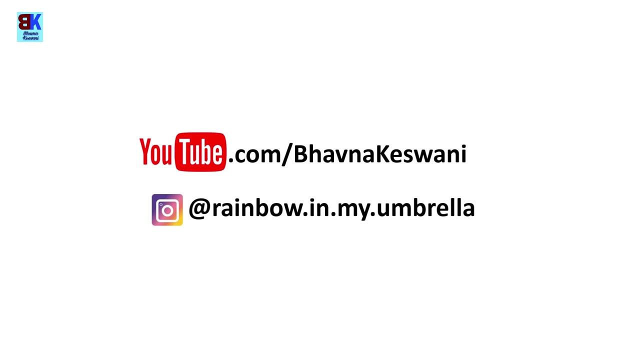 seven birds and four birds. seven is the greater number, so i will open my mouth to eat number seven. seven is greater than four. that's all in this video. i hope you understood and enjoyed learning greater than less than and equal to concepts with me as much as i enjoyed teaching them to you. 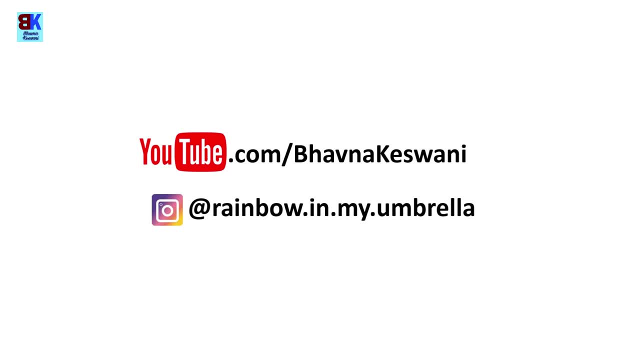 see you again very soon. until next time, goodbye, and do take good care. 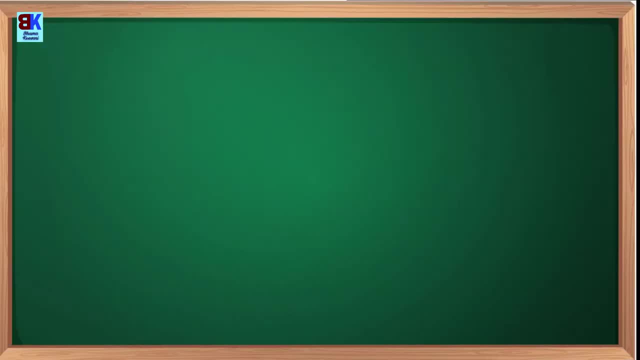 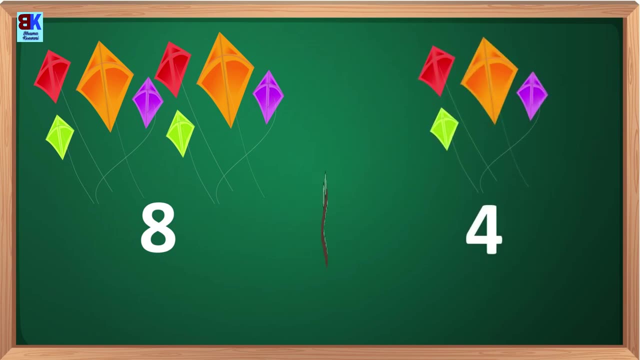 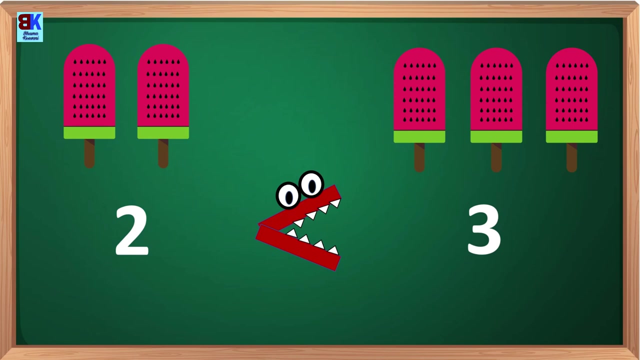 Now your turn. We have 8 kites on one side And 4 kites on the other side. That's right. I will open my mouth towards 8. Because 8 is greater than 4.. Now we have 2 popsicles and 3 popsicles. 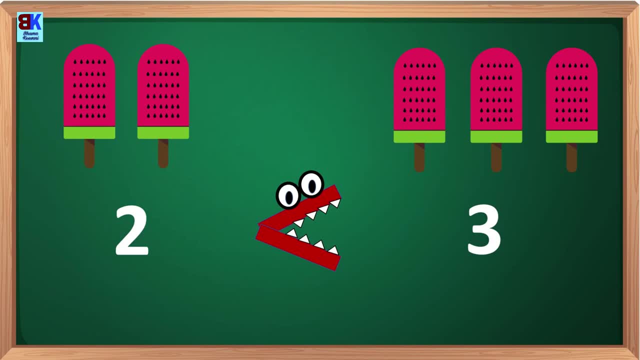 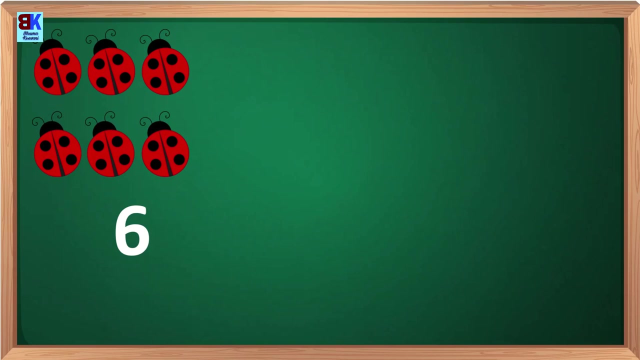 2 is less than 3.. So the back of my mouth will point towards 2. And I will open my mouth to eat the number 3, which is bigger than 2.. 2 is less than 3.. 6 lady birds and 8 lady birds. 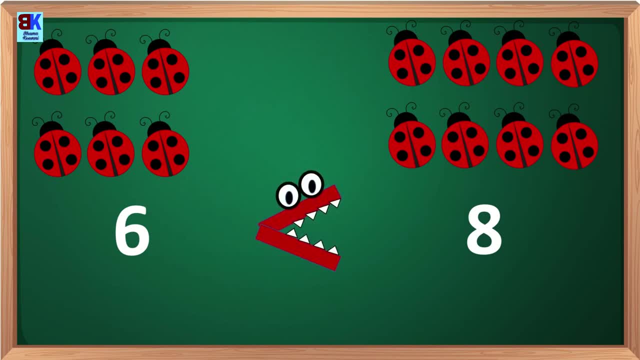 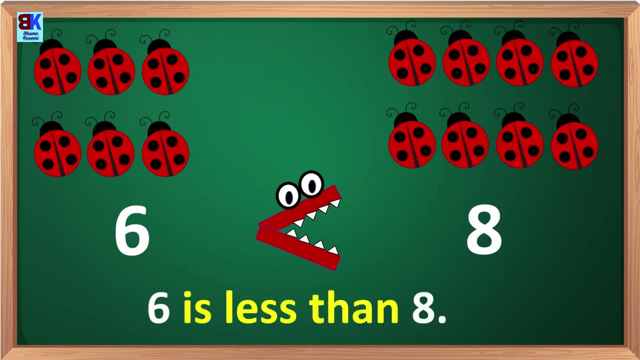 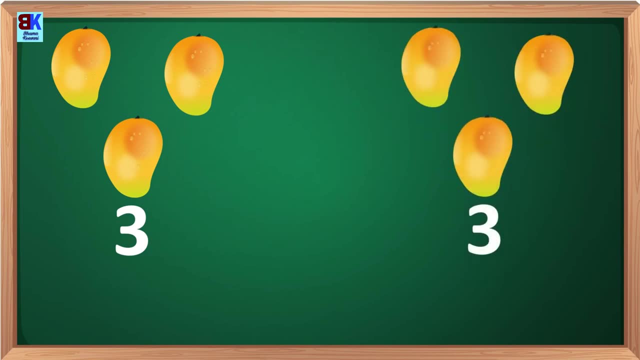 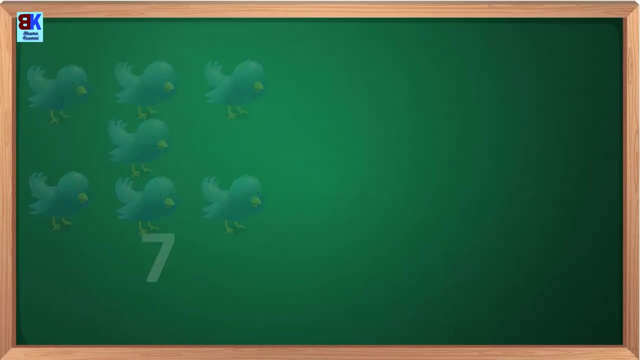 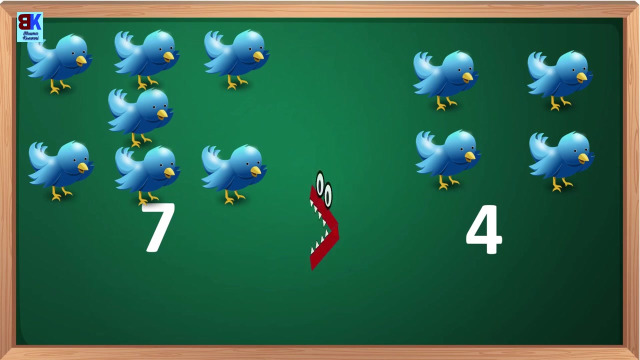 Six is less than eight. Three mangoes and three mangoes, So we have equal mangoes on both the sides. Three is equal to three, Seven birds and four birds. Seven is the greater number, so I will open my mouth to eat number seven. 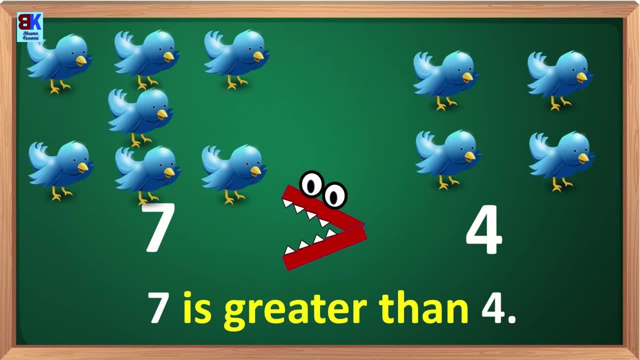 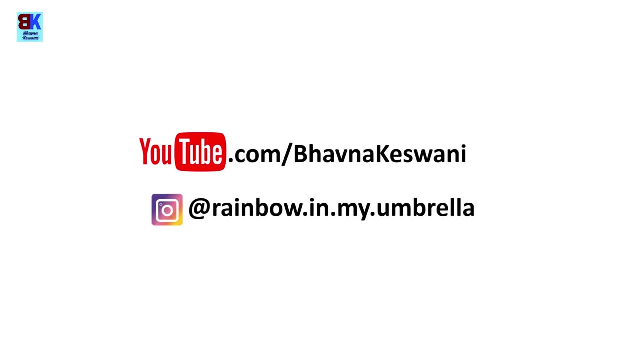 Seven is greater than four. That's all in this video. I hope you understood and enjoyed learning greater than, less than and equal to concepts with me as much as I enjoyed teaching them to you. See you again very soon. Until next time, goodbye, and do take good care.